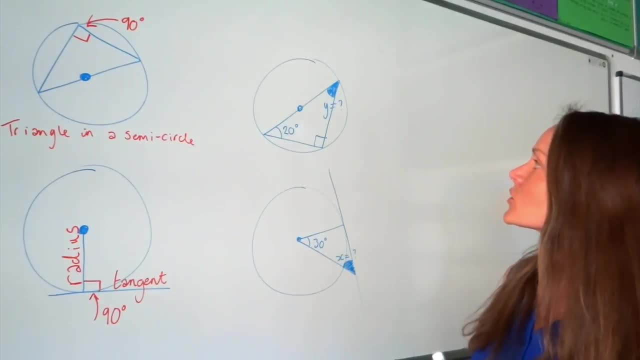 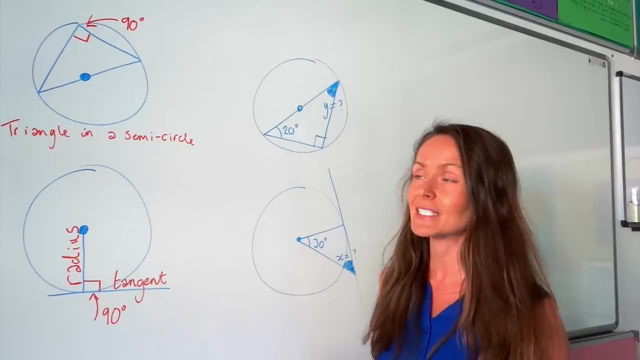 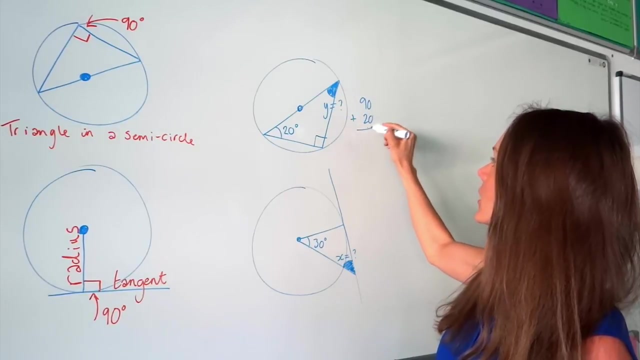 angle here is 90 degrees, this one. So we also have to remind ourselves how many degrees there are in a triangle. In a triangle we have 180 degrees, So this one is 20, this one is 90. So so far we've got 110 degrees. So to work out the 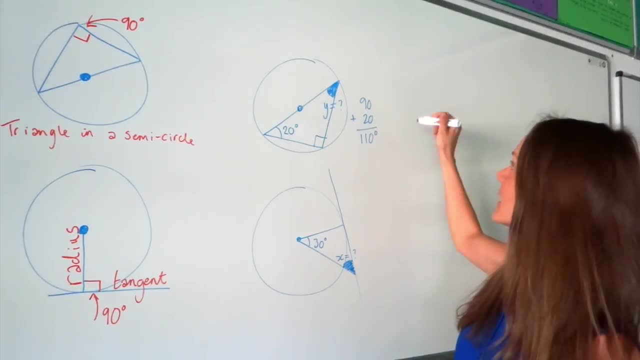 missing angle. you just need to subtract that from 180.. So when you subtract the 110 from 180, you get 70 degrees. so that is the answer to the first one there. Okay, So angle Y is 70 degrees. And if they ask for an explanation, how did you? 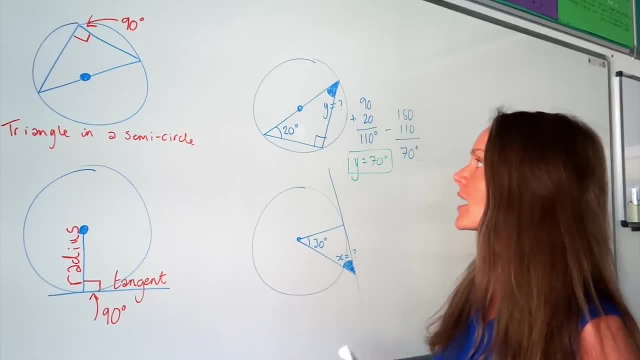 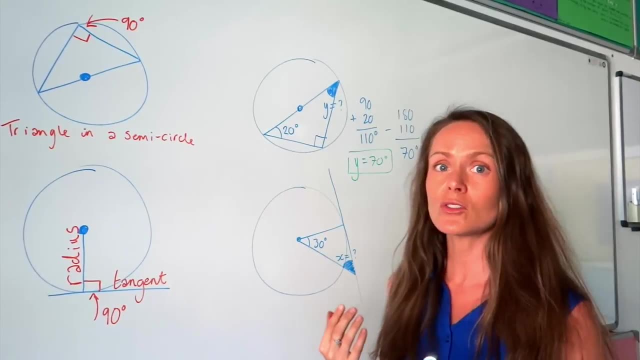 know that was 70?? Well, we use two different rules. You would say: we know this angle is 90 degrees because there's a triangle in a semicircle, and also we use the rule that in a triangle the angles add up to 180 degrees. so if you 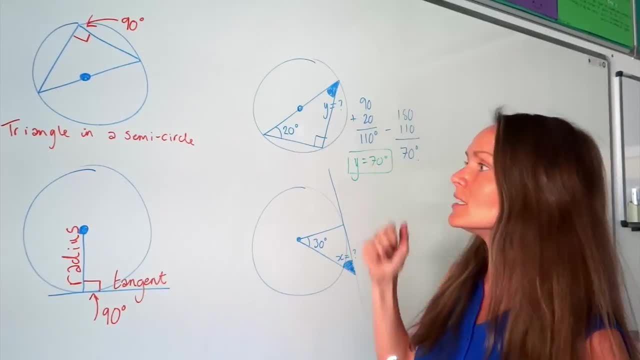 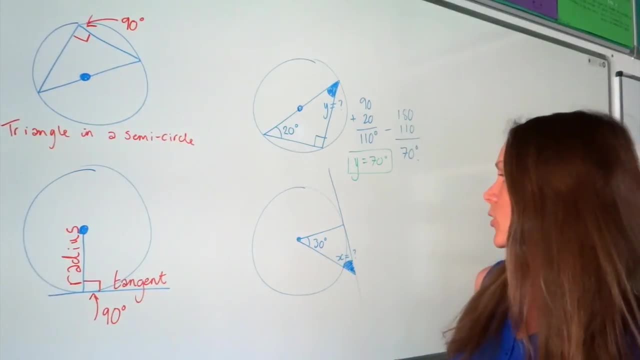 are asked to explain how you work that out. you would need to use those two rules in your explanation, as well as the calculations, which are useful too. so in the second question, I can see there's a tangent in this one. and here is the radius, so from the center of the circle to the circumference, which means we have 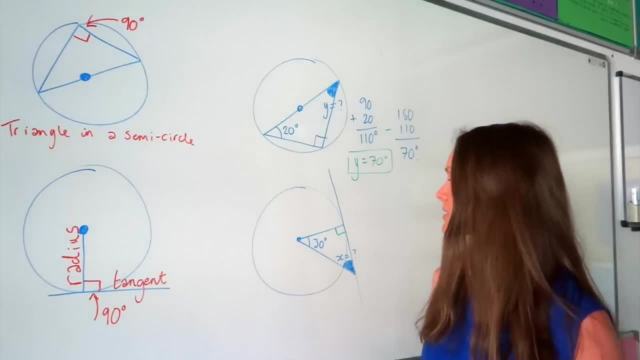 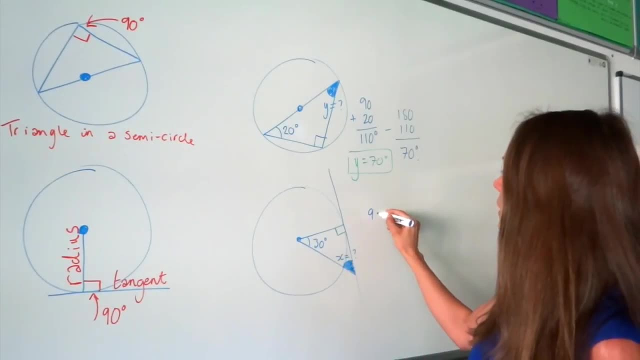 another angle there, this one which is 90 degrees, so the same as before. in a triangle, all the degrees add up to 180, so so far I've got the 90 here plus the 30 over here, which leaves me with 120, but we need to find this one down here. 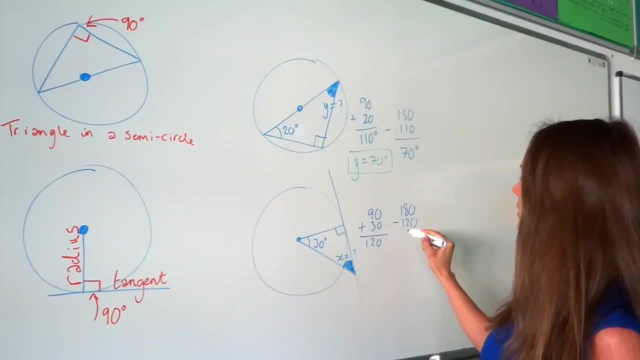 so subtract the answer from 180 to work out the missing angle. so that means the value of X is 60 degrees. so that means the value of X is 60 degrees. so subtract the answer from 180 to work out the missing angle, so that means the value of X is 60 degrees. 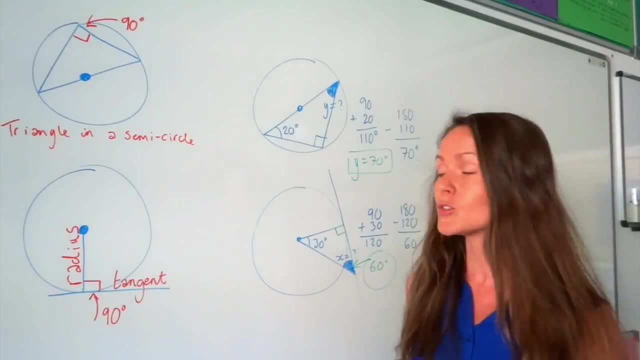 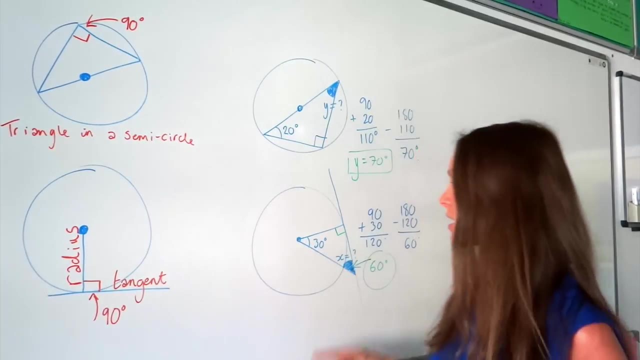 okay, and just like in the last one here, if you're asked to explain, then you would need to explain. the angle that the tangent and the radius make with each other is always 90 degrees, and angles in a triangle add up to 180, so there are a. 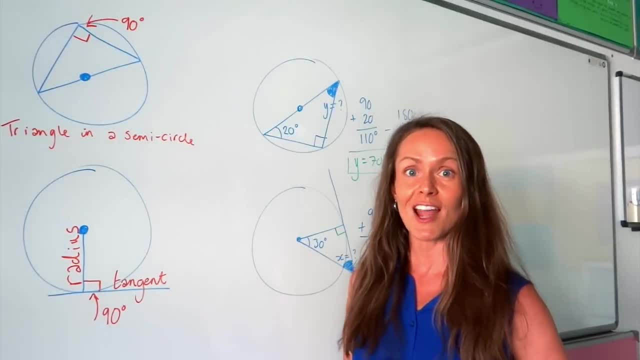 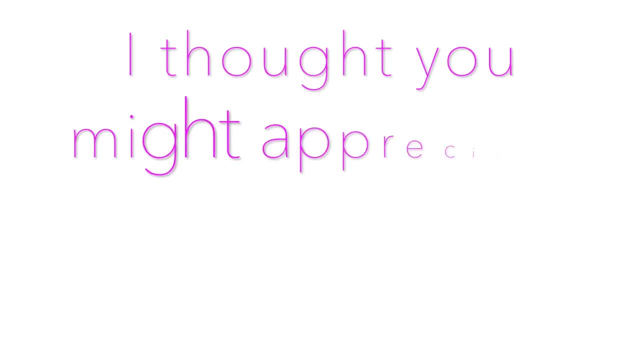 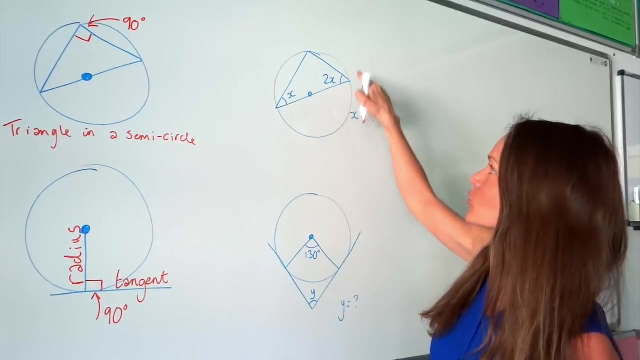 couple of easy examples. I'm going to have a go at some harder ones just now. so in this next example here I'm using triangle in a semicircle. again you can see there's a triangle in half a circle. this is the diameter, which means this: 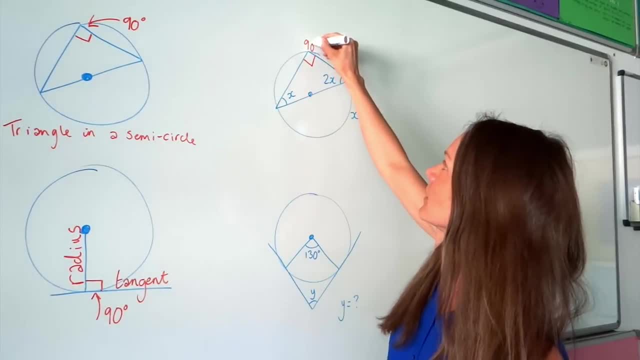 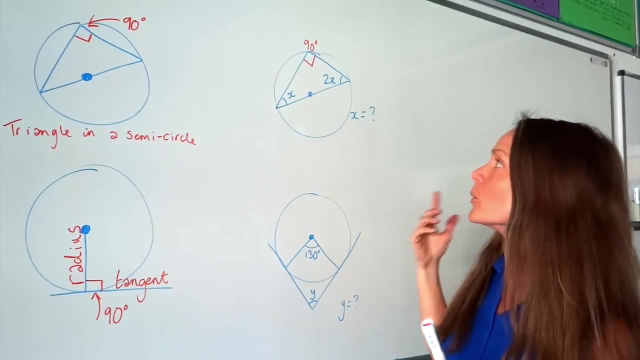 angle at the top is 90 degrees. now we need to use algebra and we need to form an equation in order to work out the value of X in this question. we know that in a triangle, all the angles add up to 180 degrees, so we can use this fact to write. 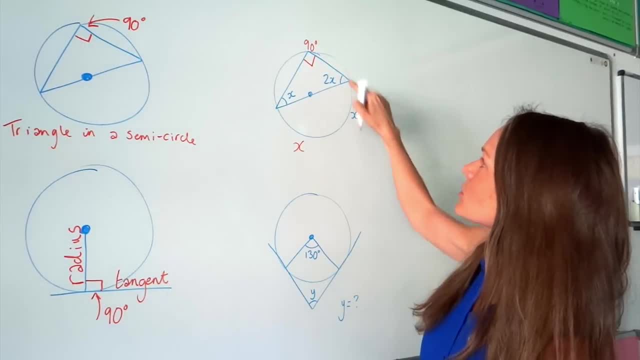 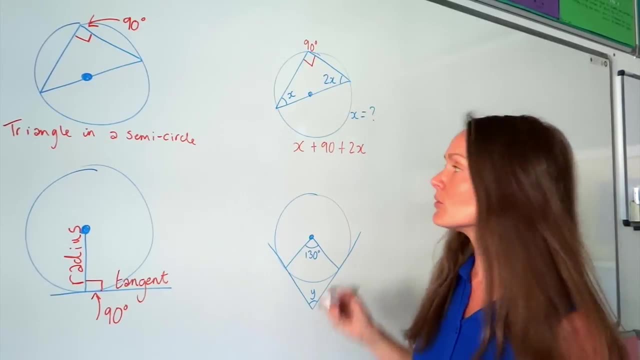 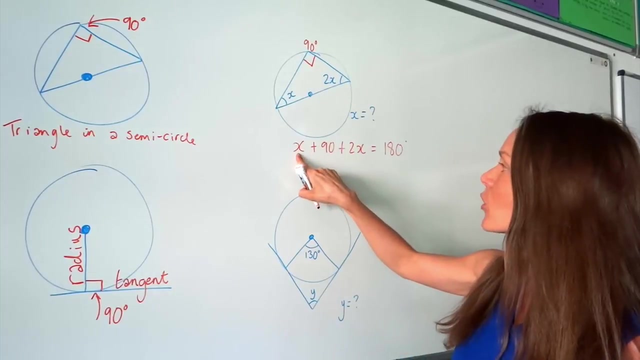 down an equation: if I add together all of these three angles, so X plus 90 plus 2x, I know, if I add those three together it should give me 180 degrees. now I'm going to simplify this and then solve the equation. here I've got 1x and I am 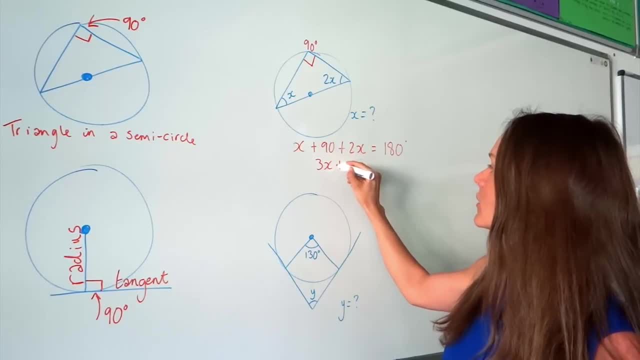 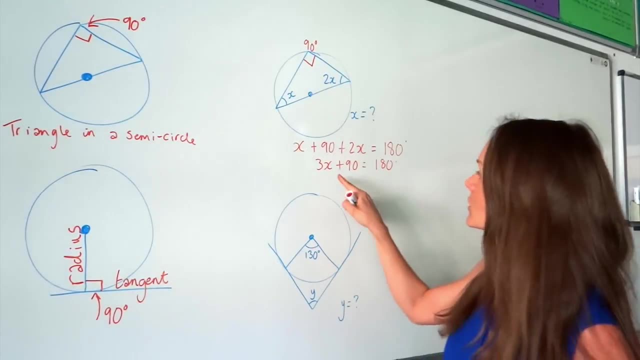 adding 2x here, so that gives me 3x, and then I've still got plus 90 and 180 still over on the right hand side. so remember, when you're solving linear equations you need to reverse all of the operations around X until X is by. 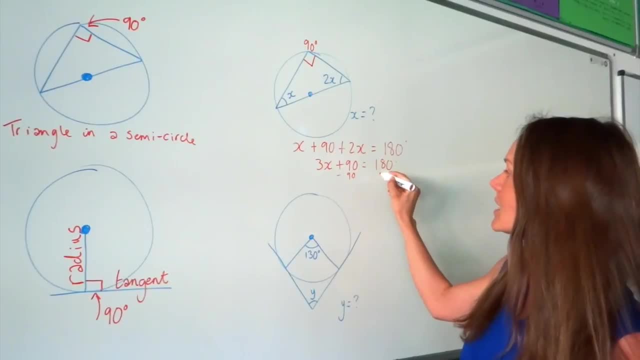 itself. so I'm going to start by subtracting 90, and remember to do the same thing on both sides of the equation. on the left hand side, that just goes to zero and I'm left with 3x, and on the right hand side, I'm left with 90 degrees. 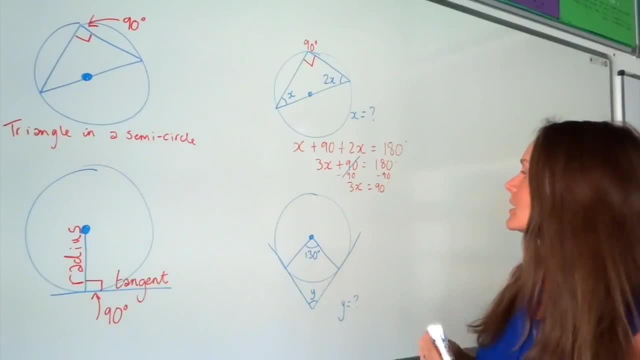 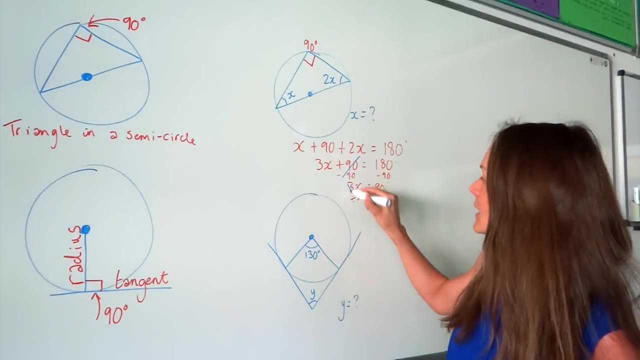 so the last step is to remove that 3. so I need to divide by 3. remember to do the same thing on both sides of the equation. so 3 divided by 3 leaves me with 1x, and on the right-hand side, 90 divided by 3 is 30 degrees. so I've 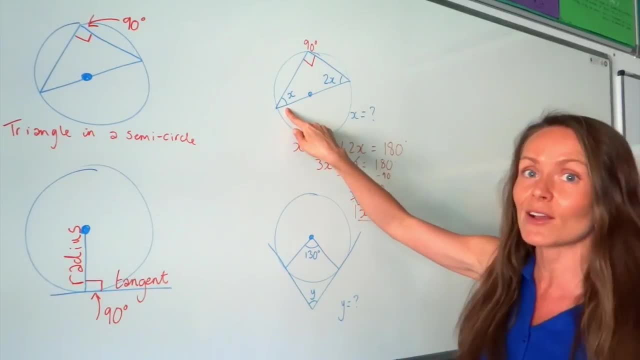 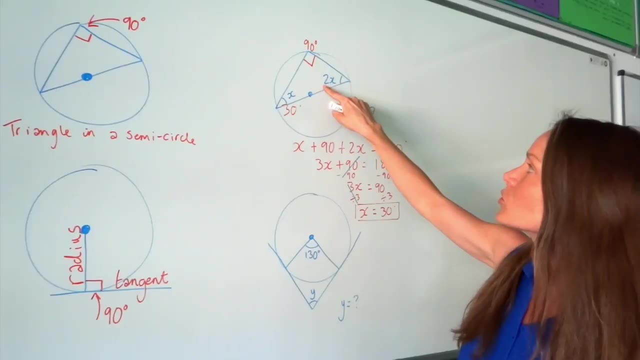 solved that equation and I found the value of this angle here, so this one up here is 30, and if they ask you to work out what this angle is as well, well, it's just 2 lots of X ¯. 2x 0, 0.